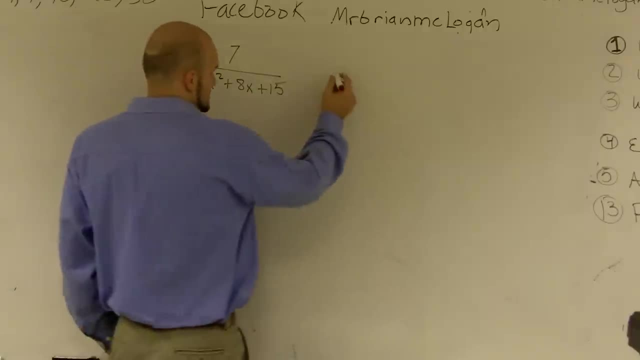 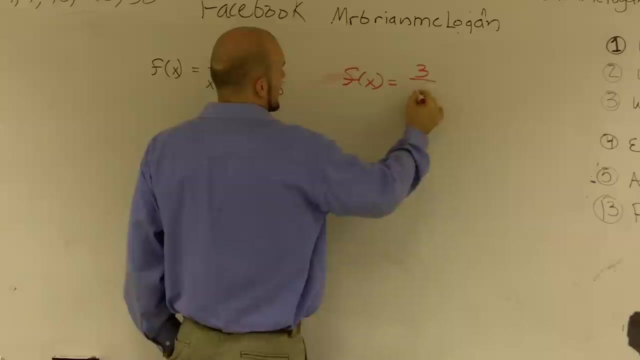 and there is no output value. For instance, let's just say I did f of x And if I did 3 over x, well, the only value that this does not work for is when x is equal to 0. Because when x equals 0, I have 3 divided by 0. 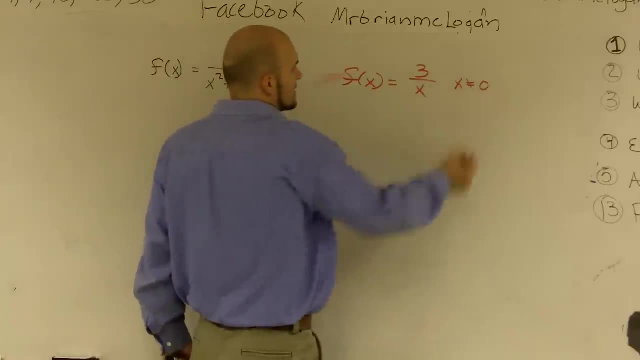 And you cannot divide 0 into a number. So therefore we write: x cannot equal 0.. So the domain for this function, if I was going to write the domain, it's going to be all real numbers, all numbers, negative 5, negative 13,, 107. 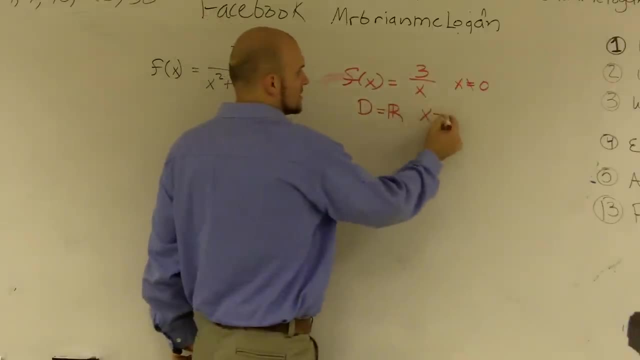 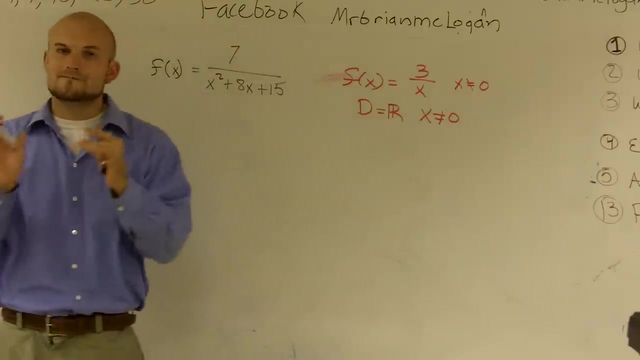 All numbers work except for 0. So when we're trying to find the domain of a rational function, what we want to do is we want to find out what values make it 0 on the bottom. So here I have a quadratic Expression. 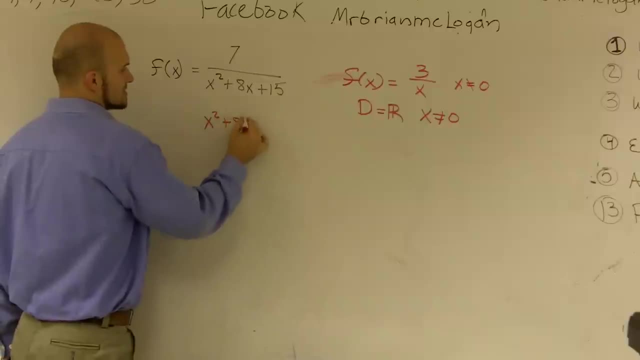 So I need to figure out: x squared plus 8x plus 15 equals 0.. I want to figure out what values can I find for x that are going to make this function 0. So when we have a quadratic it's a little bit difficult. 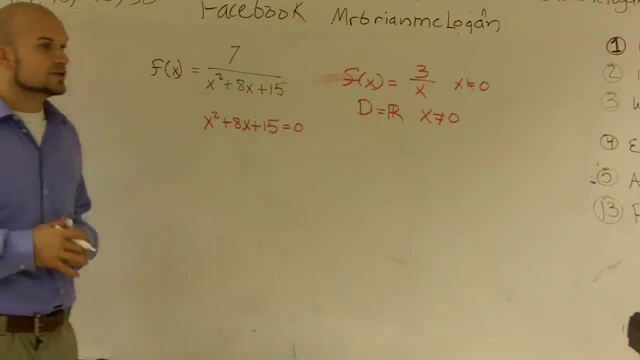 It's not like a regular linear equation where you can just solve for x. We're going to have to do some type of either squaring or factoring. Since I have two x's, I know that I'm going to want to do factoring. 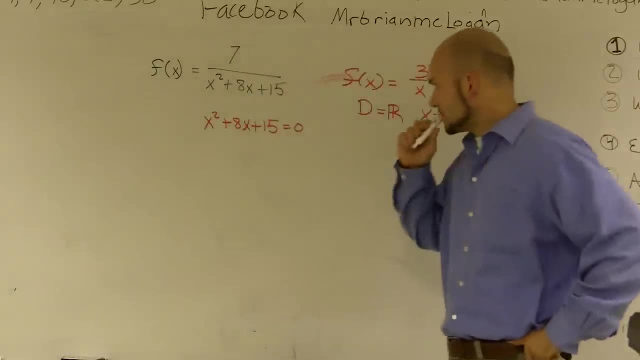 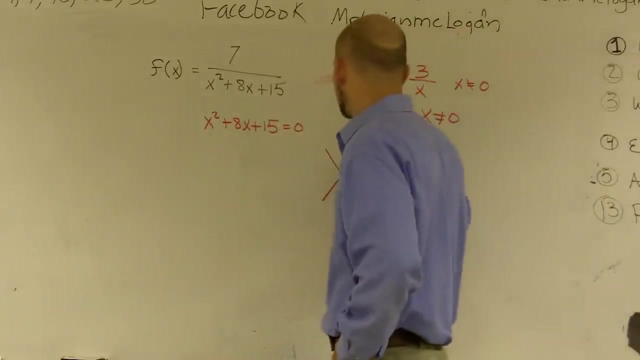 So what type of factoring do I want to do? Well, here, my a is equal to 1, b is equal to 8, and c is equal to 15.. So a lot of times, what I'll do is I'll just take my a times c, which is 1 times 15,. 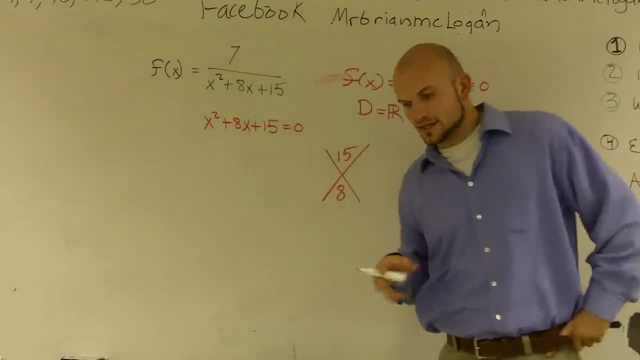 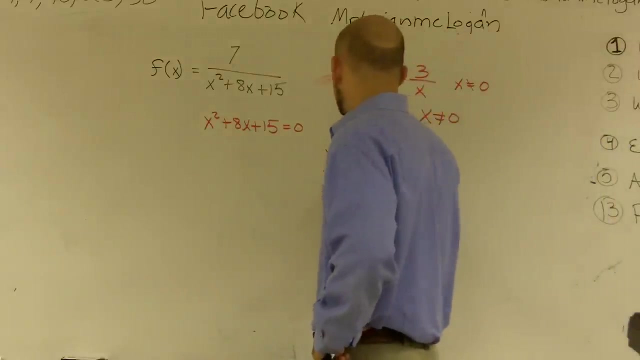 and I'll take my b, which is 8. And I'm just going to systematically think of what two numbers multiply to give me 15, but add to give me 8.. And those answers are going to be 3 and 5.. 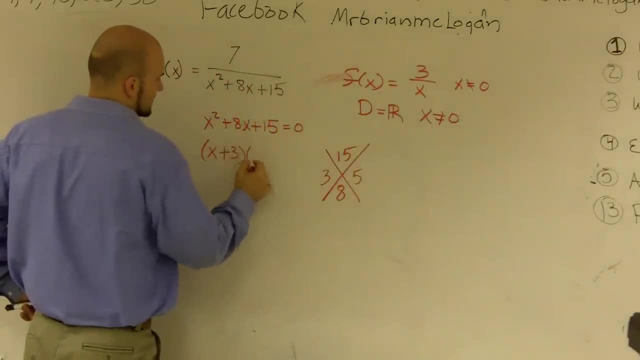 So, therefore, I can factor this to be x plus 3 times x plus 5.. And if I was to FOIL this back out, I would get this expression: Now: either one of these multiply to give me 0.. So, therefore, one of these has to be 0..